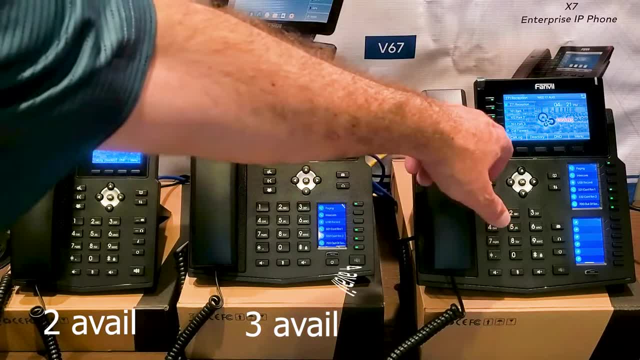 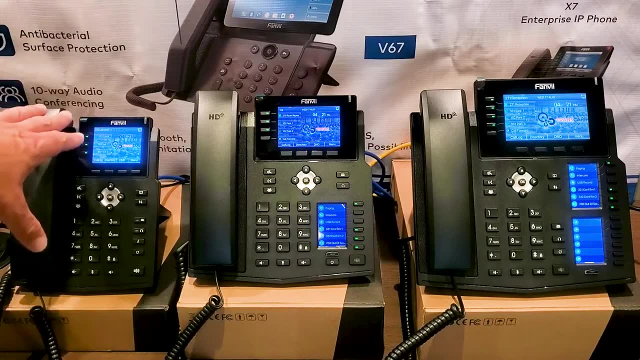 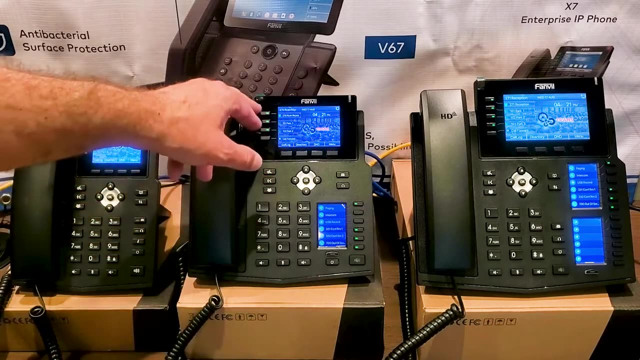 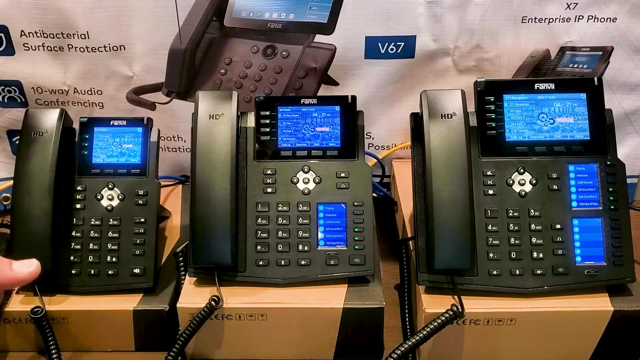 two available buttons here: three available on this one and four available on this one. Usually we are using parking spot keys for those buttons, so this is almost always consumed with your line key plus two parking spots and there's no extra room for additional programmable buttons. and on here we do the same thing: line key, two parking spots, and now we have an extra button we can do something customized with. so on this phone we put a call forward button. 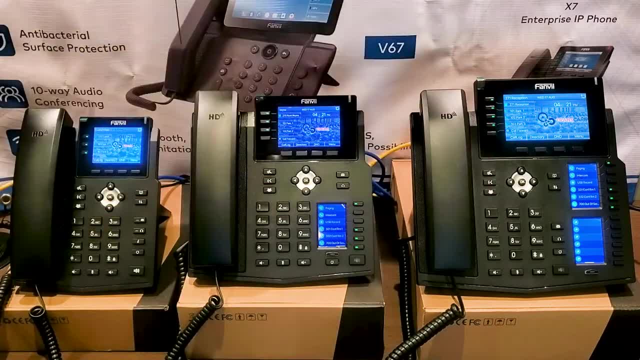 Over. on this one we have even more spots available, so we decided three parking spots. Another main difference between this one and these two are kind of the speed of the UI. Maybe it doesn't matter to some people, but it matters to me. 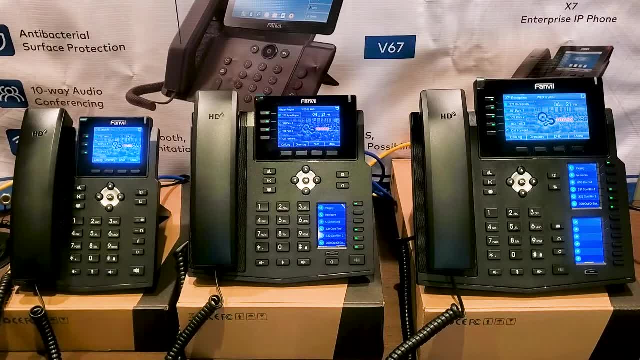 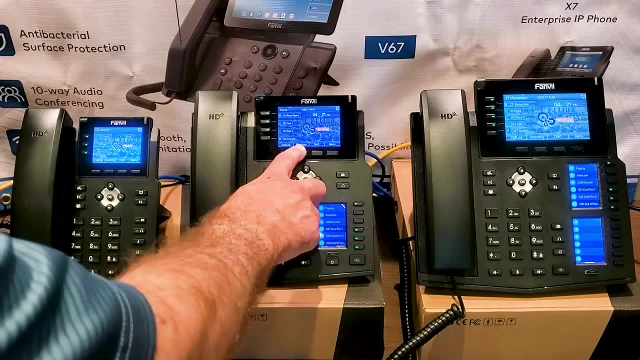 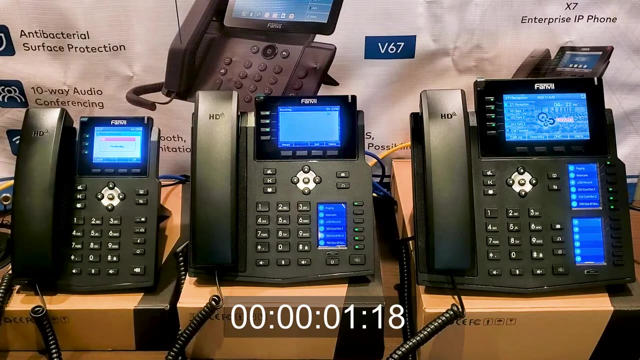 and this phone is a little bit more sluggish due to just a more economical CPU that they put in that phone. so just to give you a visual demonstration, I'll push the directory button on both phones at the same time and you'll see which one responds faster. One, two, three go. The race is on All. 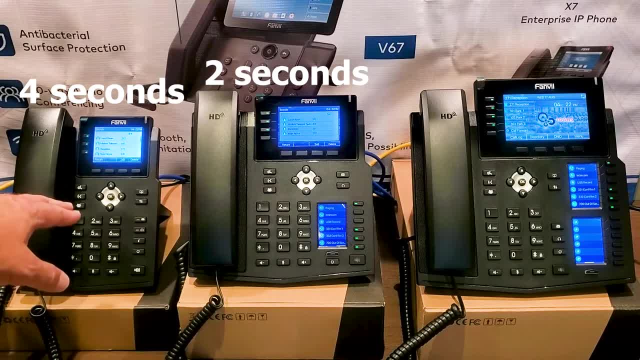 right directory definitely came up faster on this phone and only just now came up on that phone. so just to give you a little bit of an idea, I'm going to push the directory button on both phones at the same time and you'll see which one responds faster. 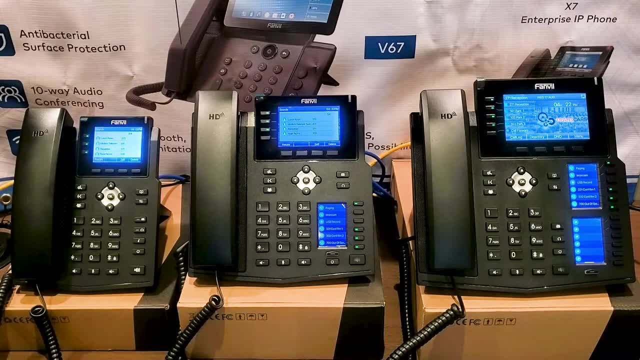 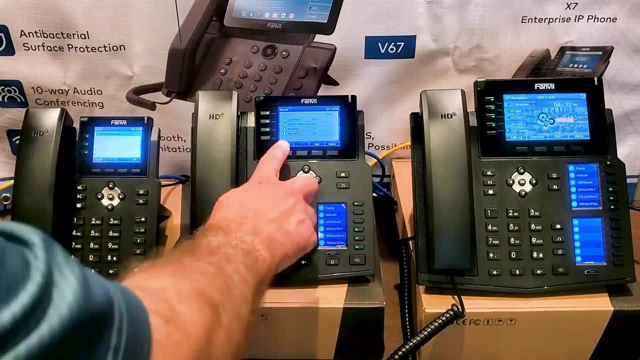 Just day-to-day use of some of the features. if you're going to be using company directories, navigating your call history or going through menus of the phone, these ones are going to be faster, I believe. if we do the same race with these two, I think it'll be the same. Let's see. 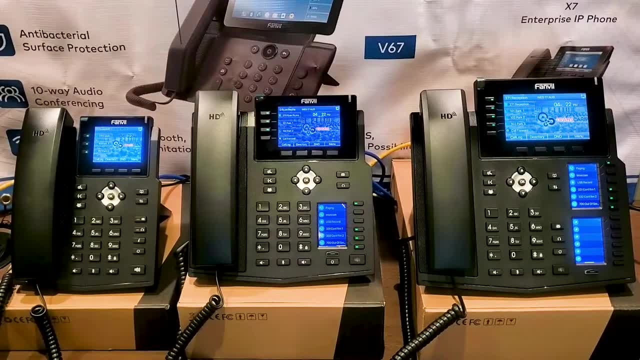 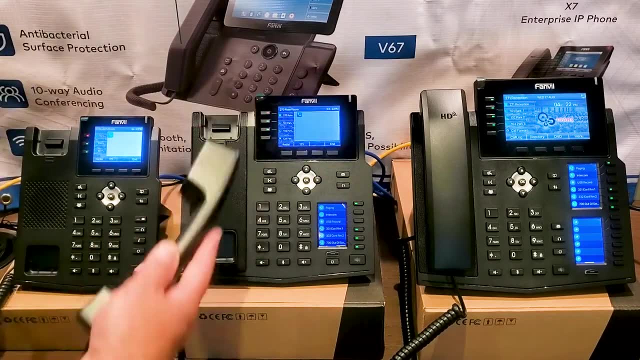 Yep, so those two are about the same, as I suspected- Sound quality. so they- all three phones- are going to share the same handset, so when you're talking on one of these doodads, you're going to have the same experience. 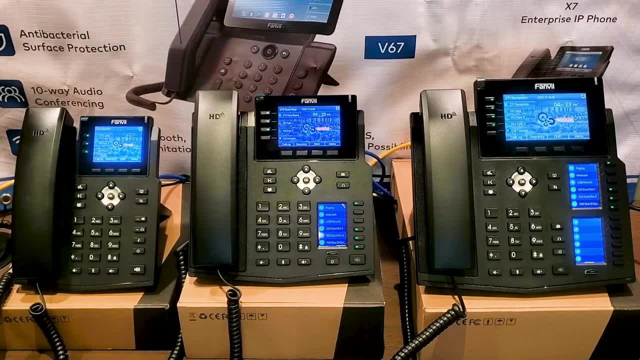 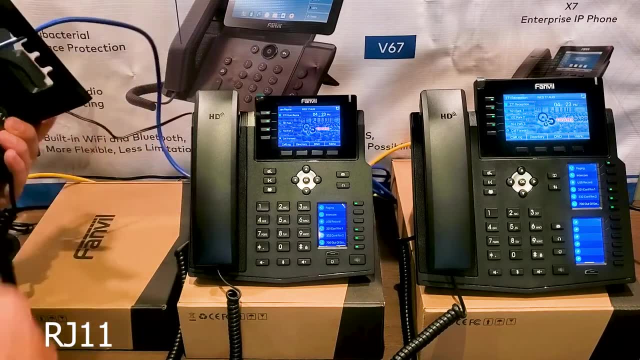 If you are using a plug-in headset, your options are more limited. So on this guy you can only use an RJ11 style, which is the traditional style headset plug-in which goes into a port on the back, similar to the curly cord that's running the handset. 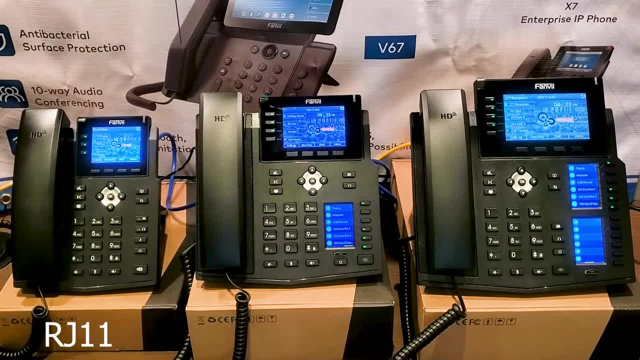 All right. on these two model phones you actually have two additional headset options you can use. There are USB ports on the backs of these two model phones- so the X5 and the X6, you can use USB headsets. There's also Bluetooth. There's also a USB port on the back of these two model phones, so the X5 and the X6, you can use USB headsets. There's also Bluetooth.